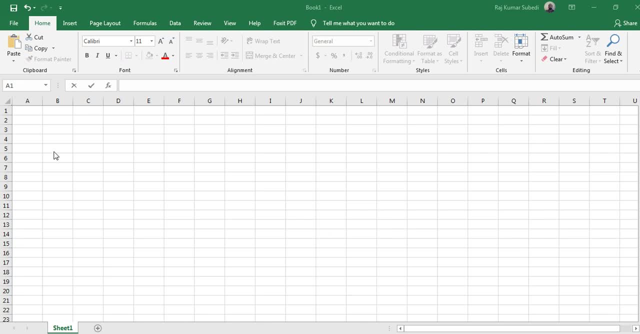 Hello everyone, welcome back to my channel. In this video I'm going to explain how to do data analysis using Microsoft Action. So Microsoft Action is very popular software. All of us might have already installed this software in our computer. So let me just directly go to the steps on how to do data analysis. 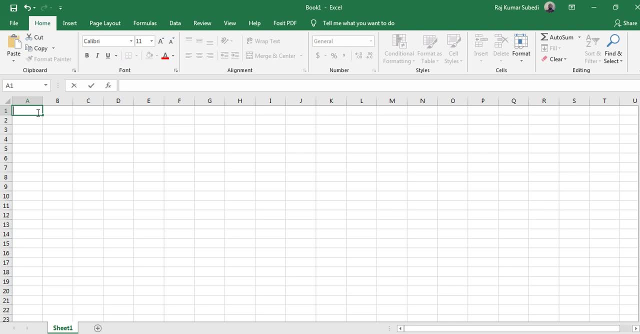 First of all, let's imagine hypothetical data. So let me enter data. okay, with some variables like serial number, gender, smoking age. okay, So let me put some data on this list. So I'm going to enter only 10 observations. So this is hypothetical data, with some variables such as the gender, smoking age. 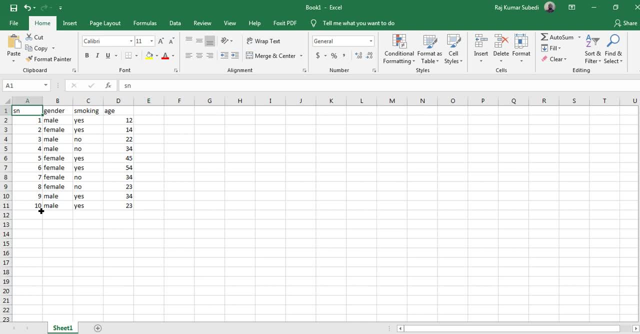 so this is the serial number, So we have the data of 10 observations. So to do data analysis, there are some tricks and tips. So first of all let me just select this section. So I selected this entire part in which there are variables and 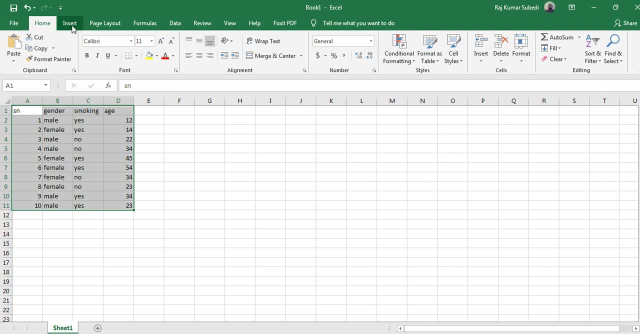 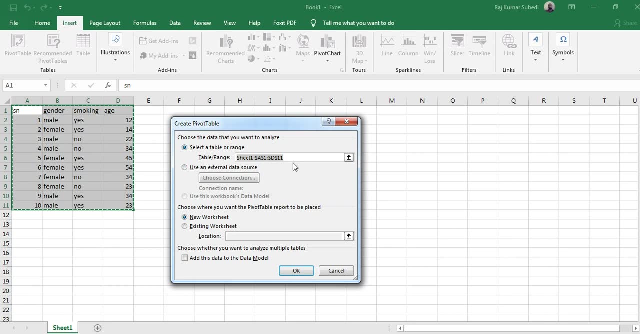 there are data. So when I select this and I go to insert and then click on pivot table, So when I click on pivot table then it displays the following dialog box: okay, So it says select table arranged. It automatically selects it based on my 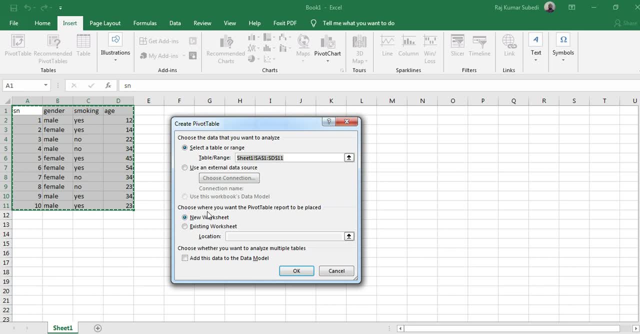 selection. Similarly, it asks us whether we want to generate the pivot table to be placed in the new worksheet or existing worksheet. So by default is new worksheet. So I don't I don't have to do anything on this one, I just click on ok. 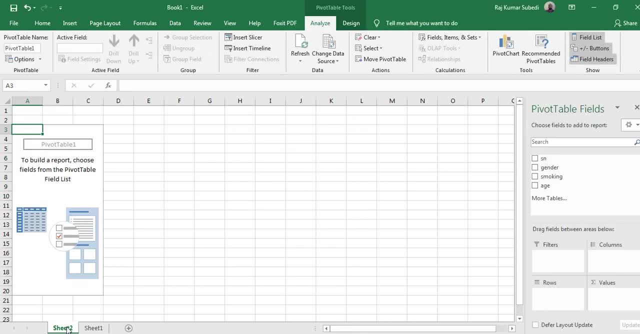 So when I click on ok, then the next seed is generated. if you see So, in seed one you have data, but in seed two you have this pivot table. okay, So when you see this seed you can see the variables in the pivot table fields. Let's say you want to. 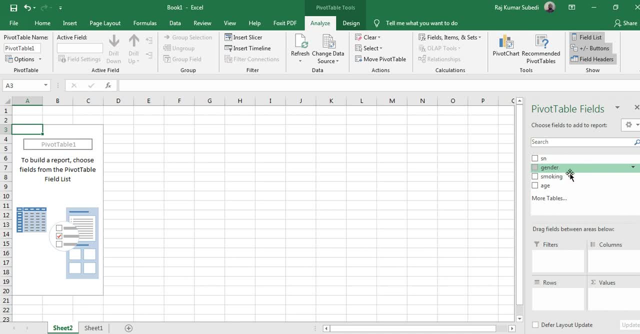 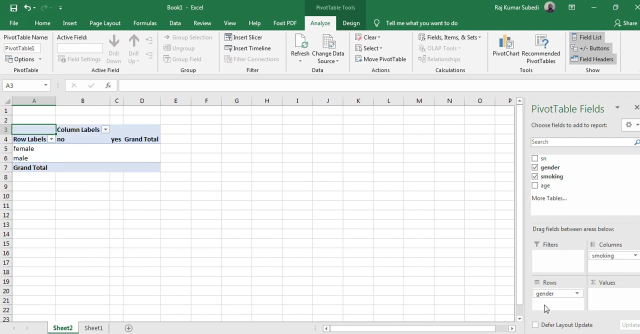 know the relationship between gender and smoking, or you want to generate cross tabulation comparing gender and smoking. So let's move this gender in row and smoking in column, So you just just drag and drop these variables in those respective rows and columns. okay, So in the values, what you can do is you can. 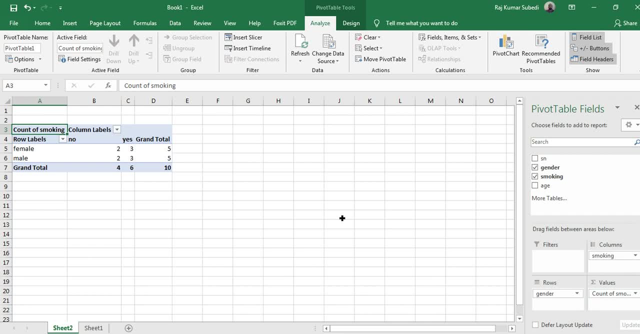 drag that smoking. So if you, if you do that, okay, you can see here the table being generated. So this was a comparison between smoking and gender. okay, So count of smoking, yes and no, and gender- male and female- So there is yes, no and total, yes, no and total. So this kind of table is very easy to 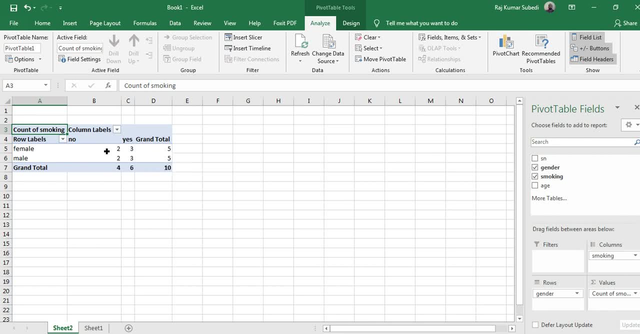 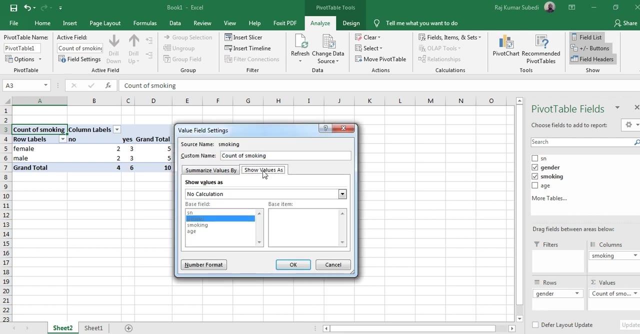 compare gender and smoking. So if you want to generate the percentage instead of numbers, then what you can do is go to this value and then click on this value field settings, Okay, and then here: so value as so in, in so value as you can select the. 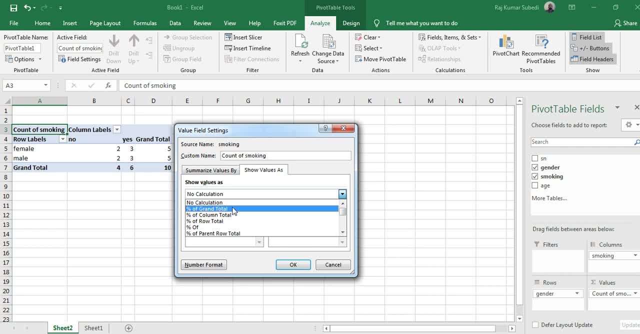 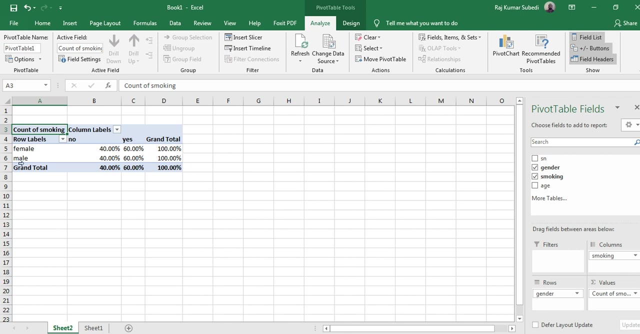 percentage. So you have to be very much careful on whether to choose percentage of column total or percentage of row total. Here we have entered gender in row and smoking in the columns, So let's select percent of row total. Okay, Click on OK. So what it does is 60% of the females were smokers and 60% of the 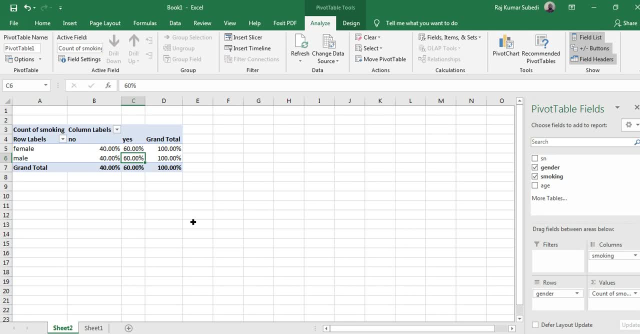 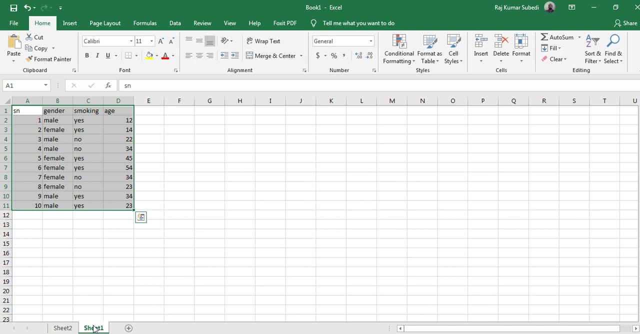 males were smokers. It generates the output in that way, okay. So based on this observation, it does the data analysis. For example, this is a cross tabulation. okay, For example, you just want to know the measures of central tendency, like mean standard deviation, etc. So to do that, you have to understand the type of 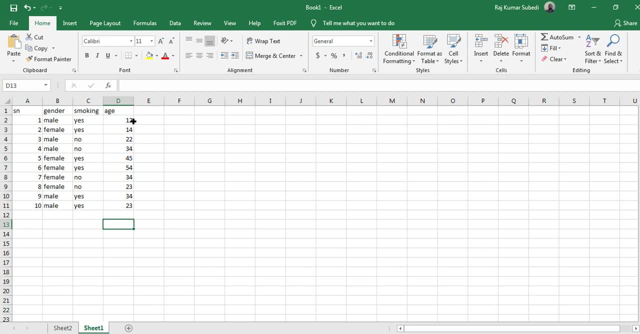 variables. You know that for quantitative data or for quantitative variable, you can calculate the measures of central tendency and measures of dispersion. Measures of central tendency include mean, median and mode, Whereas measures of dispersion include standard deviation range, etc. So let me 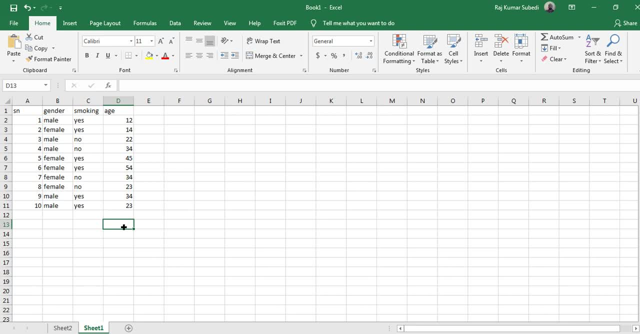 just do it very easily. So what you can do is: you can do you can type is equal to sign and then average, and then give the brackets okay and then select the data, Then close the brackets- You can see this in the formula bar as well- and then 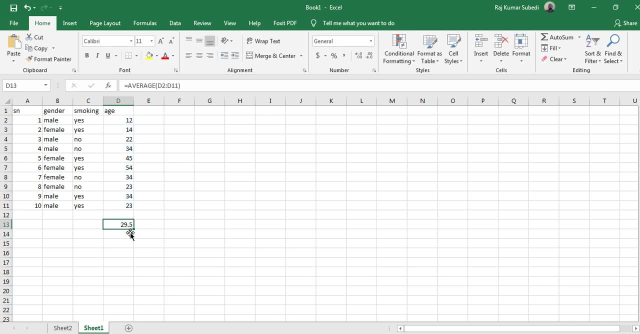 hit enter. If you hit enter, then it generates the result, which is the average of these 10 people. Okay, so the average of the mean age of the respondents was 29.5 years. Similarly, if you want the standard deviation, let's say standard deviation of this. 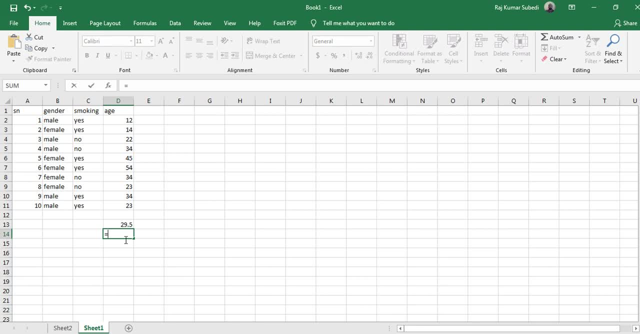 observation. then you have to type is equal to, then ESDD for a standard standard and EV is the abbreviation for standard deviation. So this is the command that Maxwell actual understands and then start the bracket, then select the data, close the bracket. you can see this in the formula bar as: 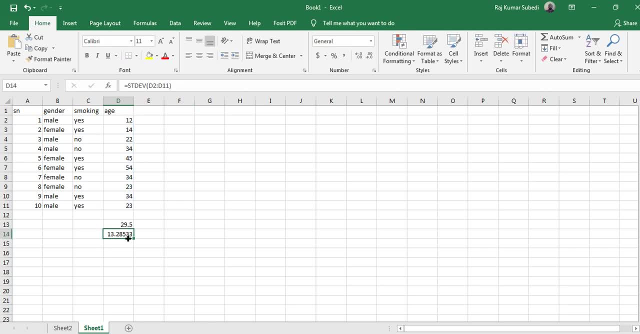 well, and then hit enter. So the standard deviation was 13.28 years, The mean was 29.5 years. So so this is the basic analysis that you can do in Maxwell. actual Hope you liked the video. guys, You can do even more. this is just the.